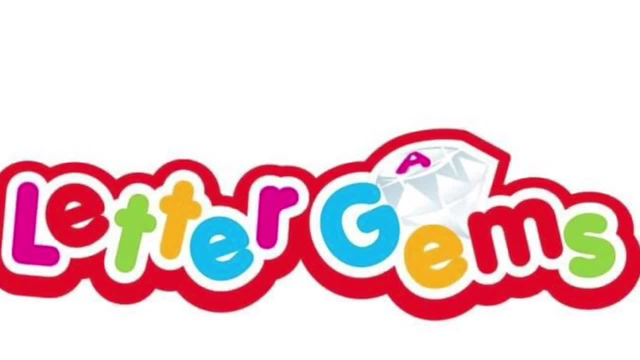 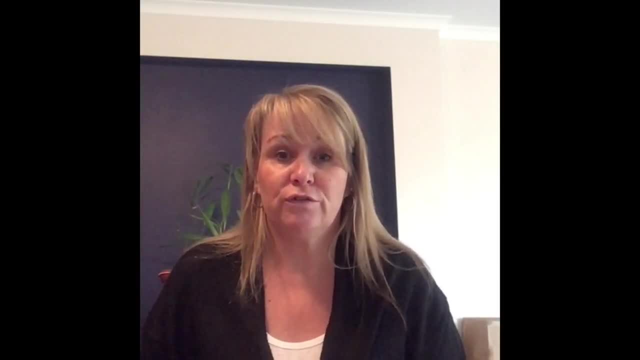 Hi everybody. I just want to spend a few minutes today just showing you a few activities to help get you through this term where we've not got current Letter Gems classes running. So I'm going to give you a few little tips on what we can be doing and I want everyone to go back to basics. 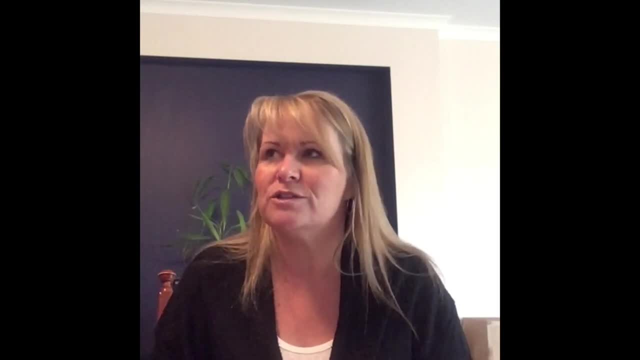 It doesn't have to be hard. I get a lot of parents asking: what can I do? I'm going to show you some really simple activities that you can do and you can leave your children alone with as well, and let them be independent learners, which is always great during this isolation period where we've got 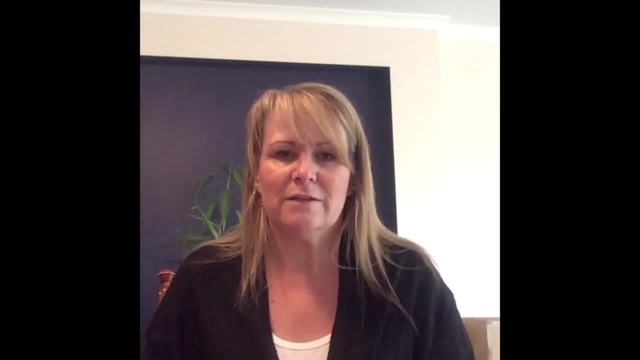 plenty to do. So have a little look at the few different things I'm going to show you. Extend upon, play with them as long as you want to, and we can change them up a little bit. So I'll try to do some indoor, some outdoor activities as well. So once we have sunshine, today's not a perfect. 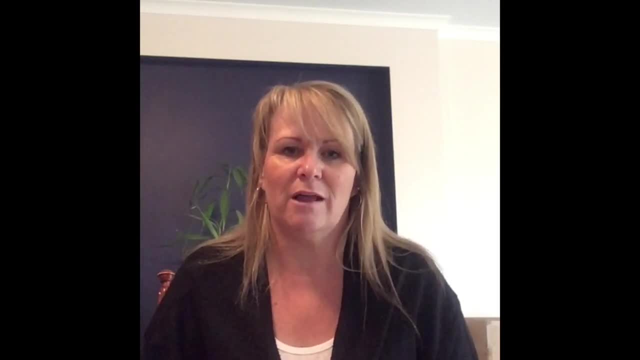 day for sunshine, but once we have sunshine, you can get them outdoors as well and they can be playing and learning. That's what I love to do. I want my children to know that they're playing. They don't realise they're learning So and that's. 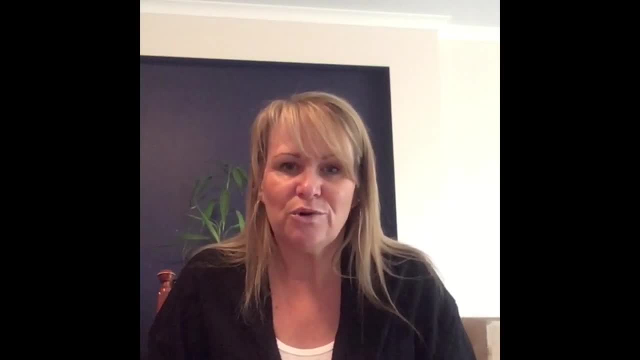 what Letter? Gems is all about making learning fun. If children see it as a chore, they don't necessarily want to partake. If they see it as fun- I'm just playing- then yeah, they're all for it. So we'll have a go and show you some activities and if you want any more details, find me at. 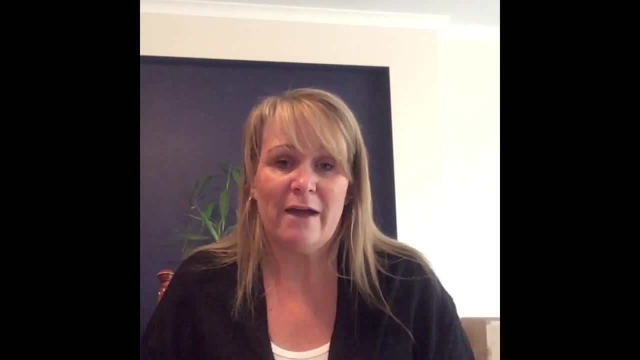 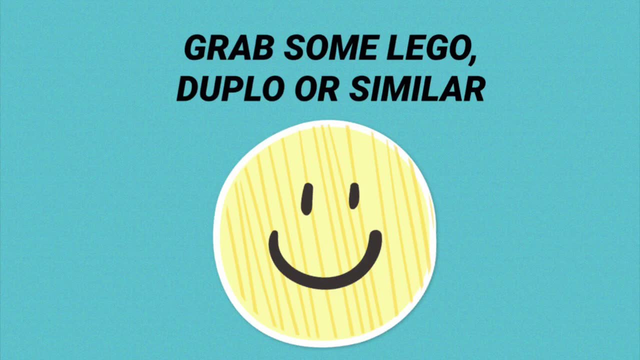 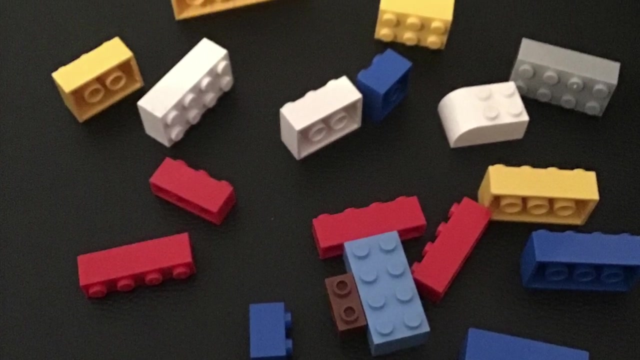 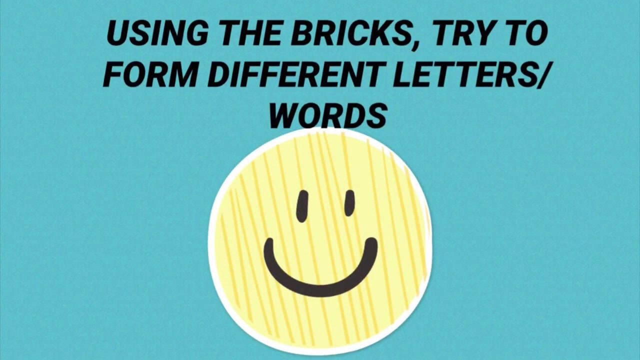 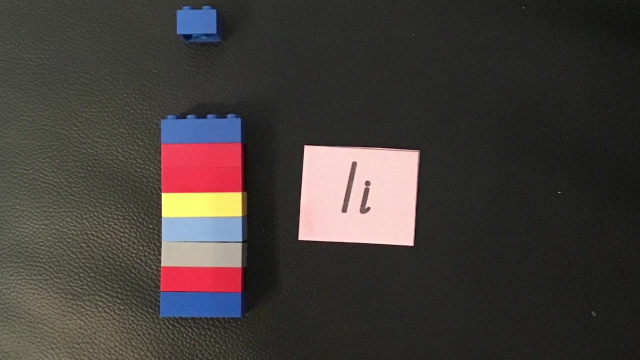 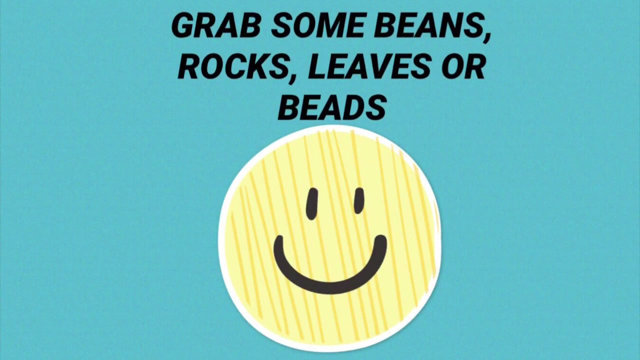 lettergems at bigpondcom or our Facebook, our Instagram page. So this one's going to go up on YouTube. Wish me luck. Thank you so much for watching. I hope you enjoyed this video. I'll see you in the next one. Bye, Bye.